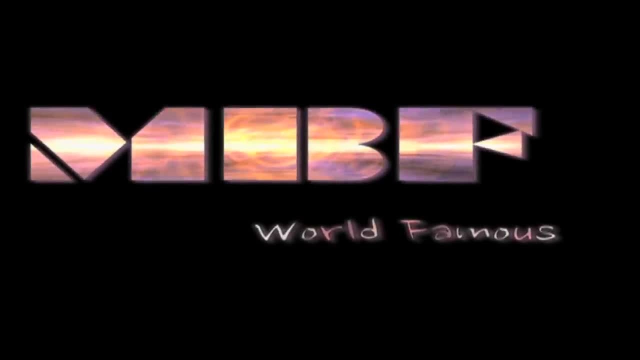 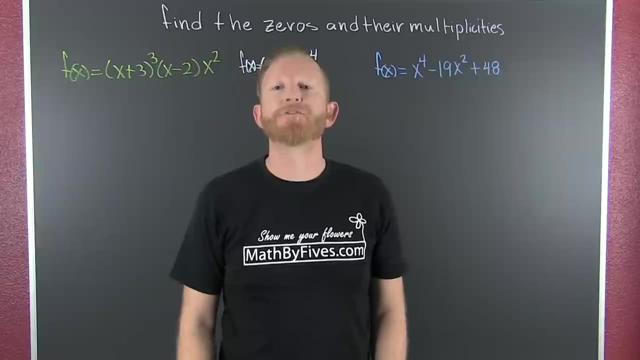 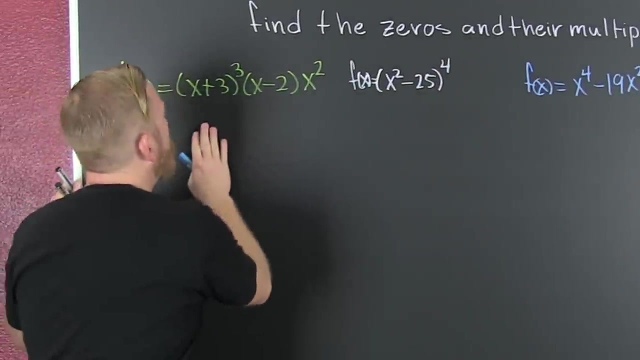 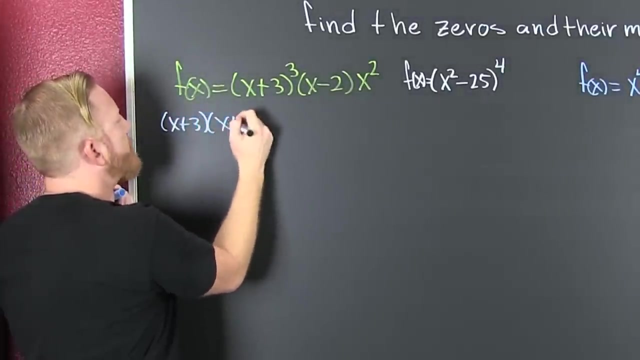 Now we're going to find the zeros and their multiplicities. We want to know how many times they occur. So we go on over here. If we're looking at this, we could write it out, We could write it. we could write it as: x plus 3 times x plus 3 times x plus 3 times x minus. 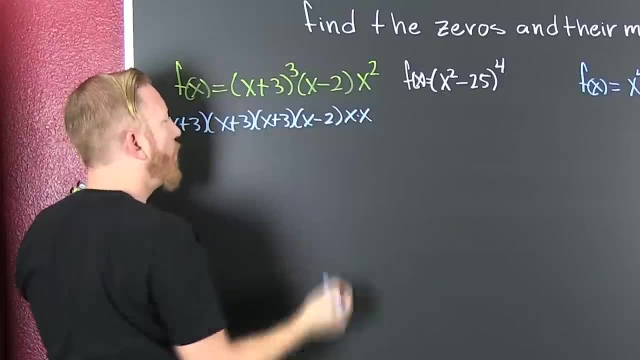 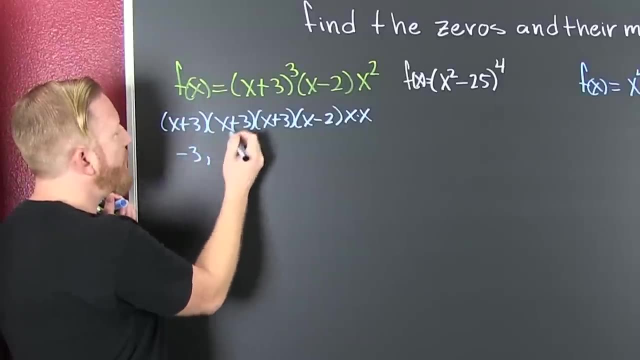 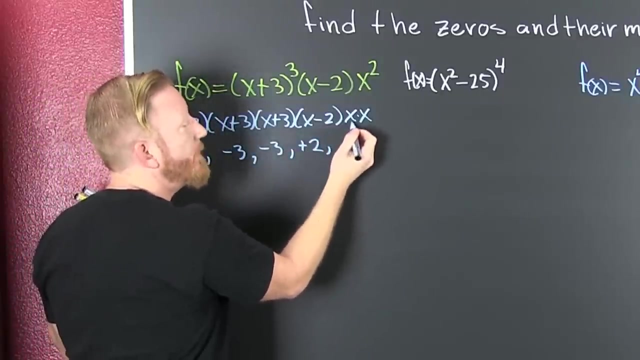 2 times x times x, Oh boy. So now that we have it all written out like that, we can go and we can find the zeros. The zero here is a minus 3.. The zero here is a minus 3.. The zero here is a minus 3.. The zero here is a minus. whoa a plus 2. The zero there. 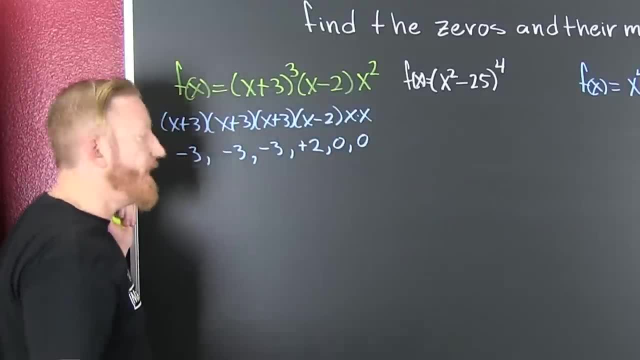 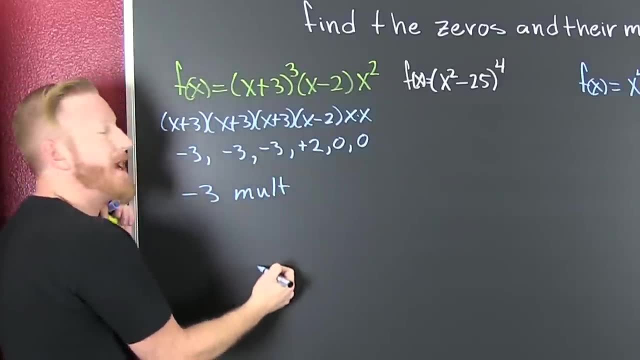 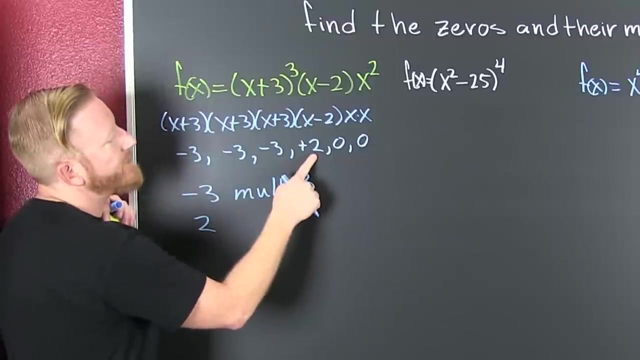 is 0. And the zero there is 0. So we can go and we can write their multiplicities: Minus 3, multiplicity what? How many times does it occur? 1,, 2,, 3,, ah, ah, ah, And then 2, positive 2.. How many times does it occur? One time? 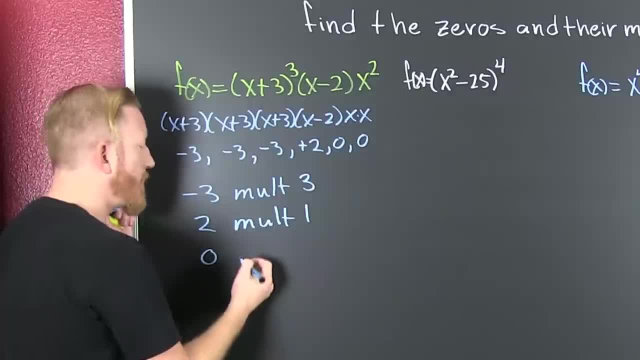 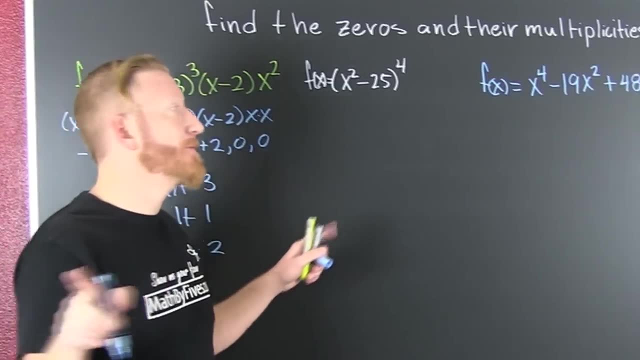 So it's multiplicity 1. And 0 is a 0 of multiplicity Deuces. Now let's go and let's do this guy over here. What if they give it to you in the wild? We need to go and we need to find. 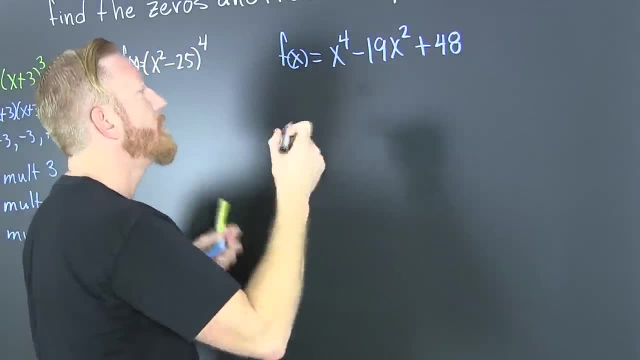 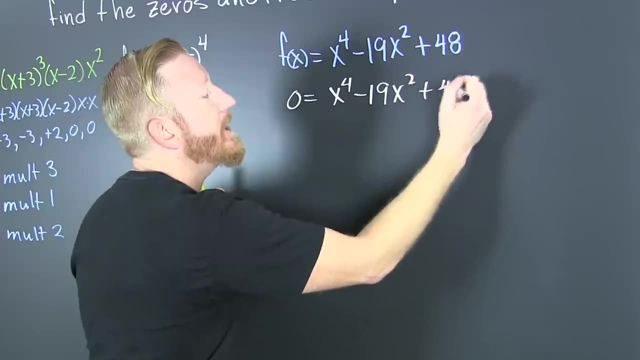 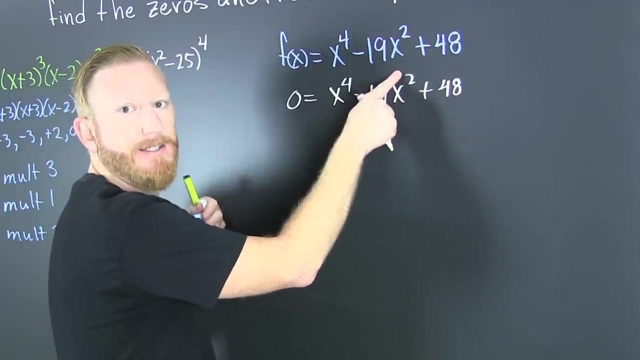 their zeros. So then we go and we set it equal to 0.. This is 0 is equal to x, to the 4 minus 19x squared plus 48.. Great Wait, This is a quadratic in form. As long as this is twice that we can factor As if it was quadratic. So then, 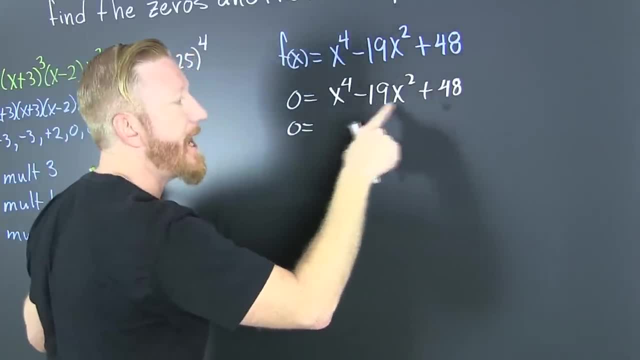 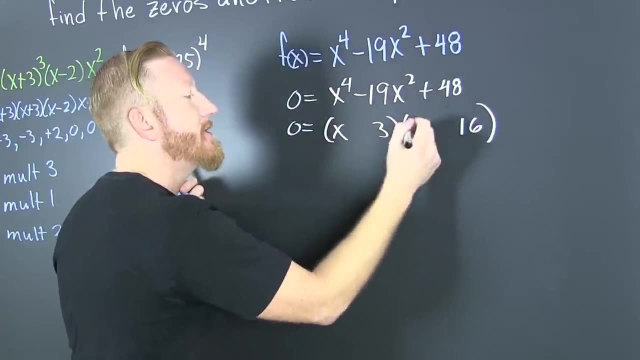 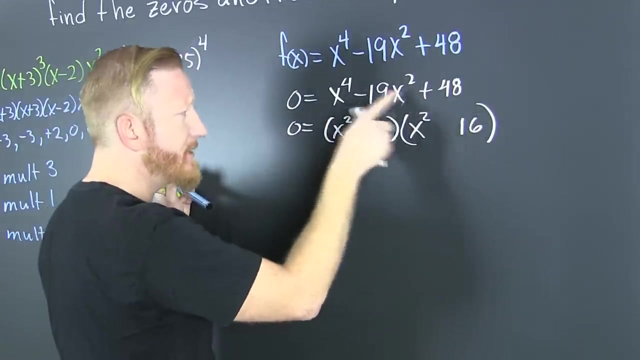 0 is equal to wait for it. factors of 48 that add to be 19.. Got to get that, Got to get that. 16 and 3.. X and x. Ah, The more the better. middle goes in there. that's an x squared and that's an x squared. so signs are the. 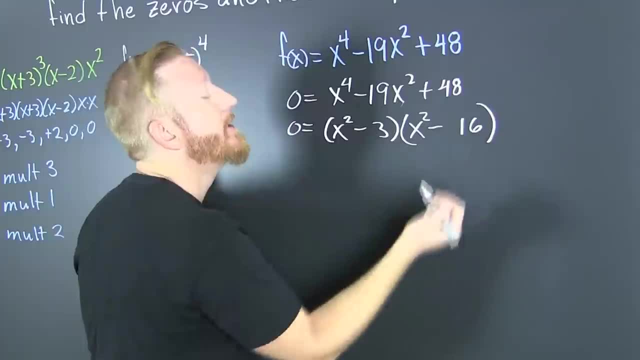 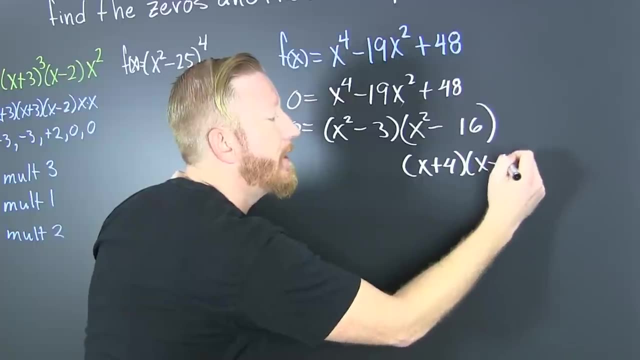 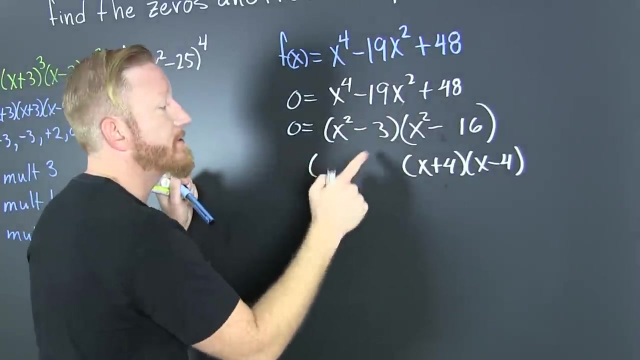 same and they're both negative. so that's a negative 3 and a negative 16. now, oh, that factors further: x plus 4, x minus 4, cuz it's difference of squares. then this one also factors. you're like, what the square, what do I square to get that? 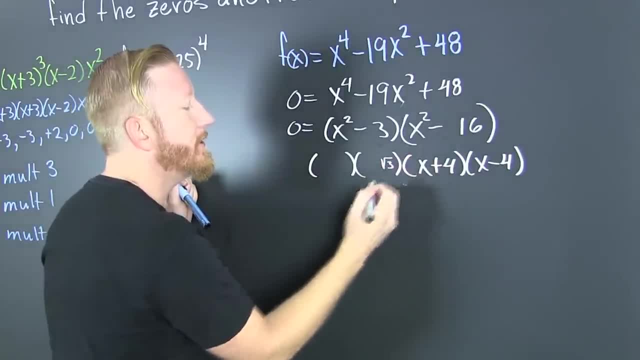 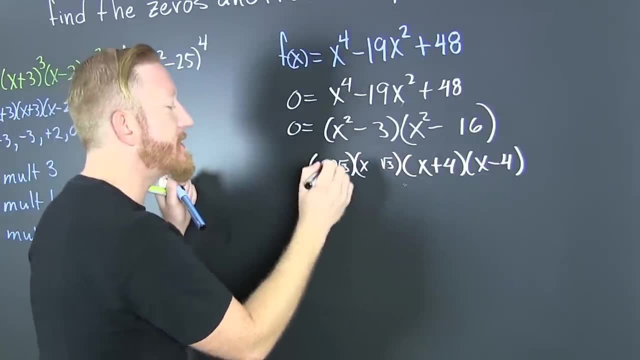 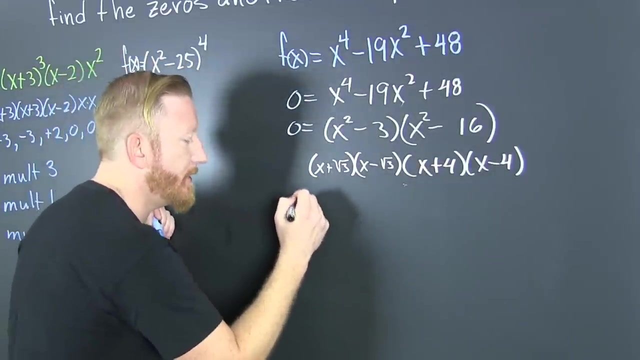 that's captured. bom, root 3, root 3, and that's X there and that's X there, and that's a difference of squares. so that's x plus root 3, x minus root 3. so here we see that our zeros are gonna be root 3 minus root 3, where the minus root 3 comes. 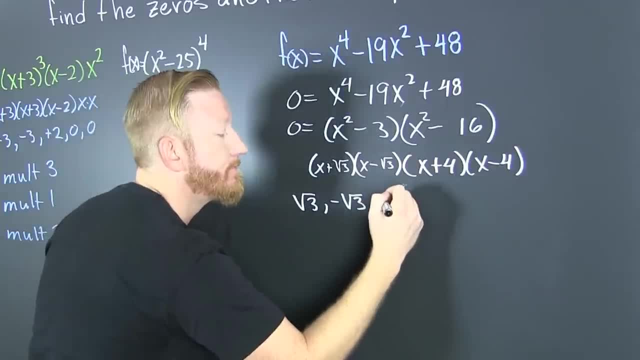 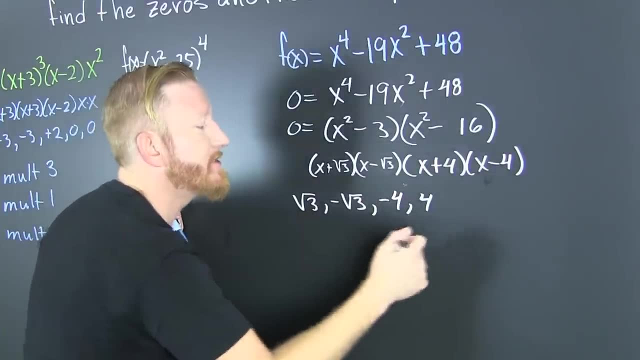 from there, and then 4 minus 4 and 4, sure, minus root, 3AAAAAA😄😏😄😏th failure. Minus 4 from here and 4 from there. So all of these are zeros of multiplicity. 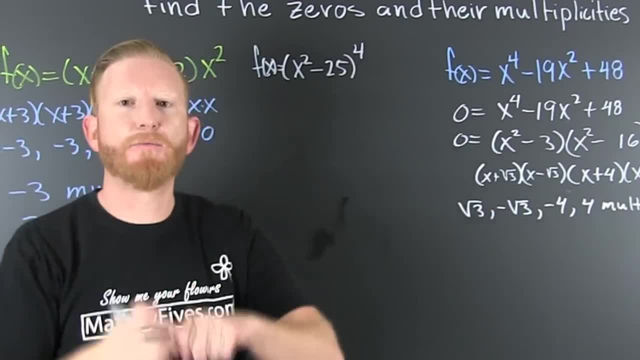 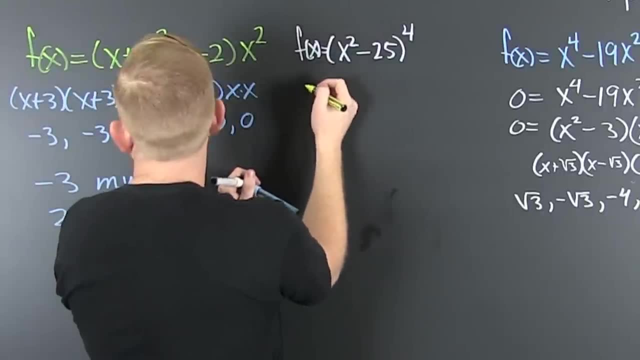 1. Let's go back to this guy: Oh boy, Uh-oh, Got factors in the middle, Sure. So then, if we're finding the zeros, boom. we set it equal to 0, and we have wait for it. 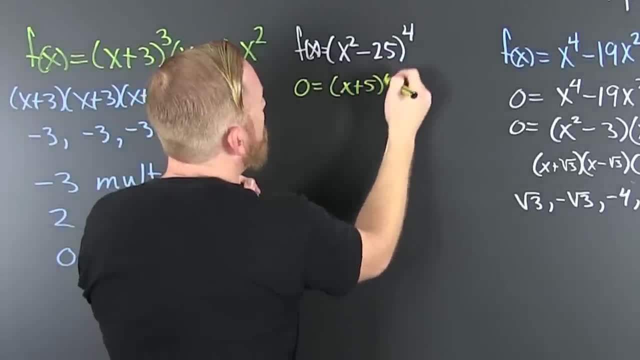 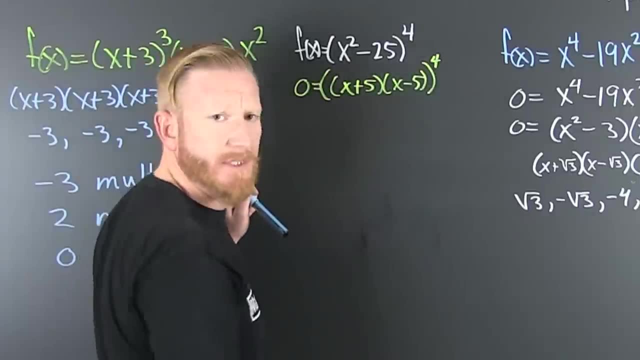 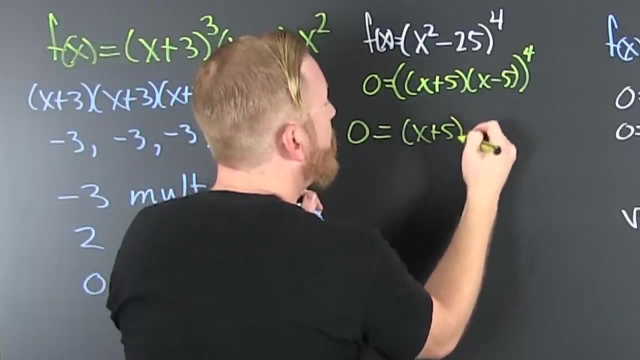 that's the difference of squares again, x plus 5, x minus 5.. But all of that is to the 4th: power. Good times, Good times, Finish him, Yeah, finish him. So this is x plus 5 to the 4th. 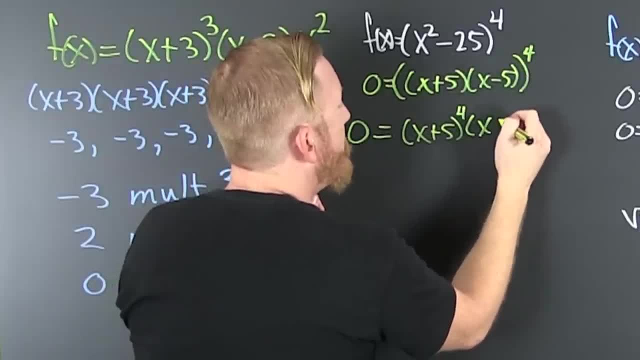 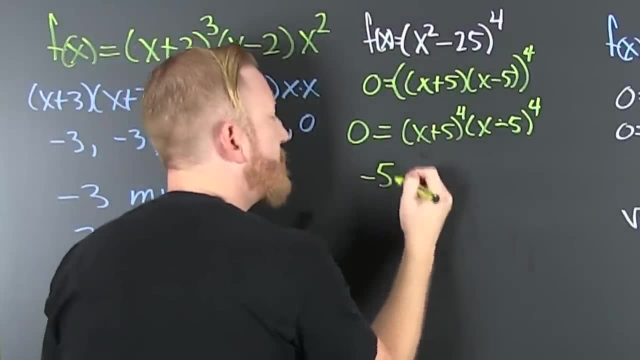 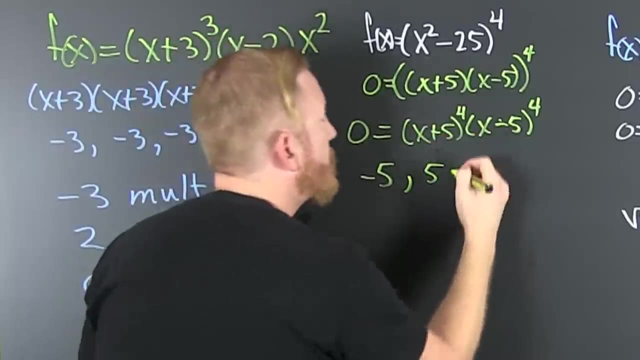 Make it rain. make it rain, And then x minus 5 to the 4th. So here we see, minus 5 and 5 are both multiplicity 4. We don't have to write it out. When I say write it out, I mean like that: 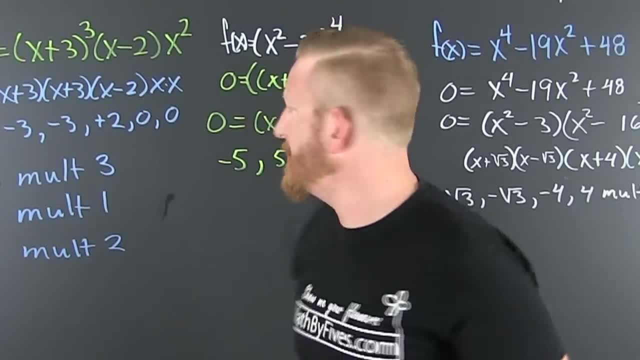 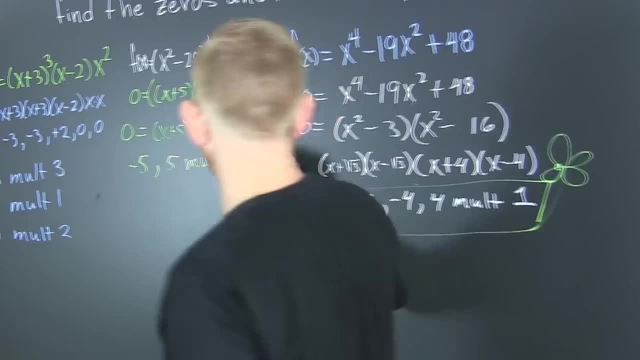 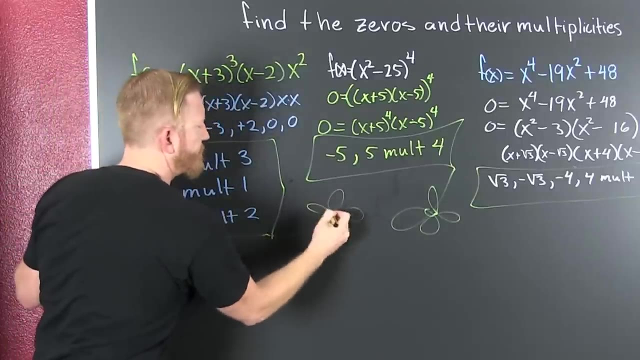 Multiplicity: 4.. Ah Box and flower Box and flower Box and flower. We're sorry, The number you have dialed is not available. dialed is not in service at this time.